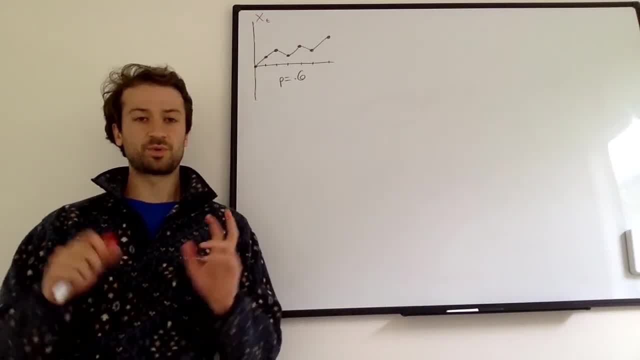 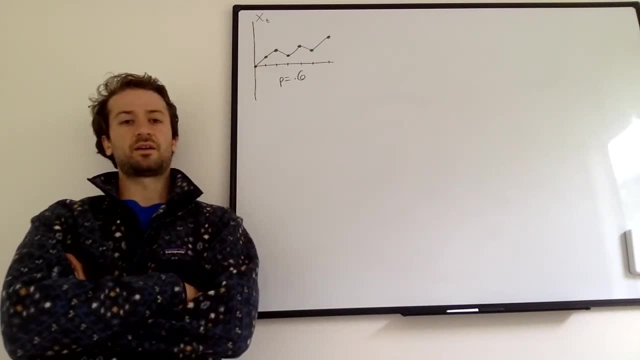 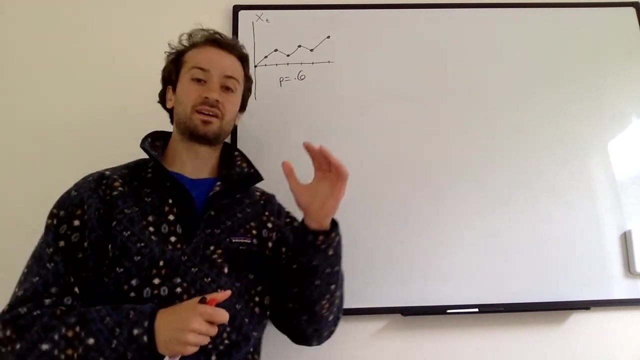 Welcome. So today we're going to be talking about simple random walks, which are stochastic processes that hopefully you're relatively familiar with. We're going to be talking about hitting probabilities, which is a term I like to kind of consider, a term I like to apply to the probability that a simple random walk will ever achieve a certain level. 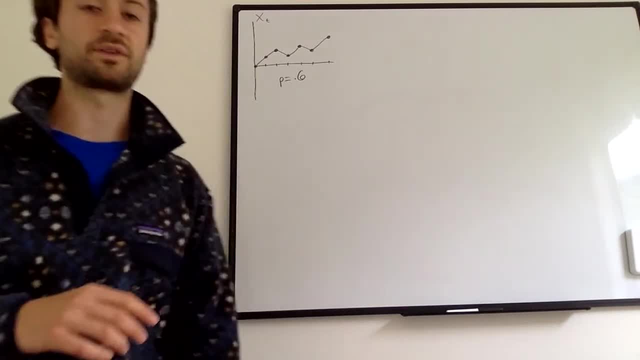 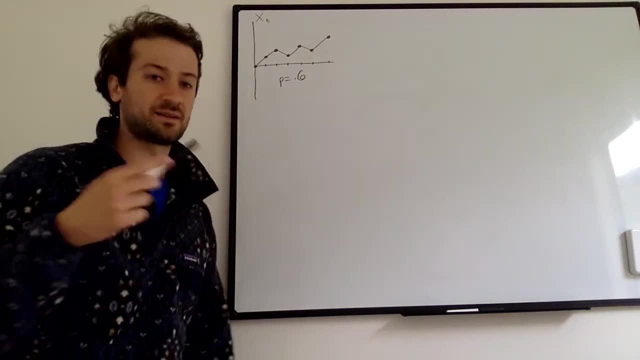 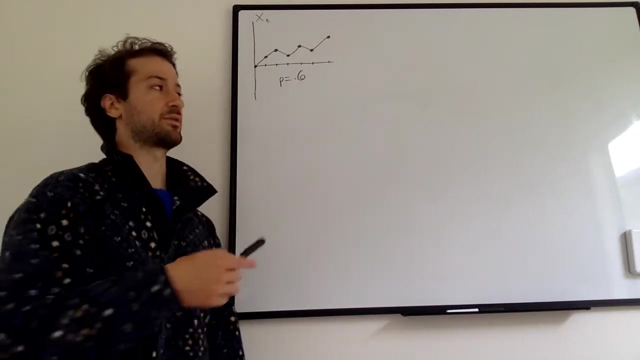 But before we do that, let's just do a quick overview of simple random walks. I've drawn one up here labeled it x sub t. The t sub t kind of indicates that this random variable is indexed to time, which is what makes a stochastic process. stochastic processes evolve through time. 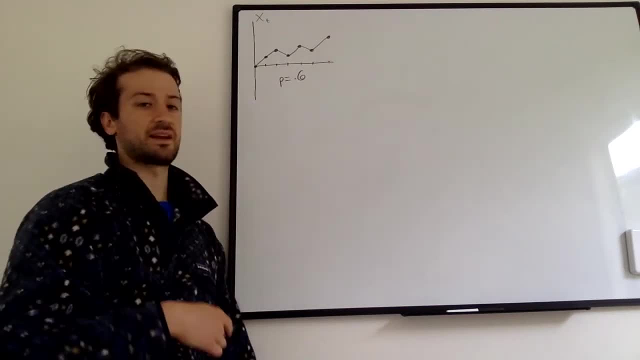 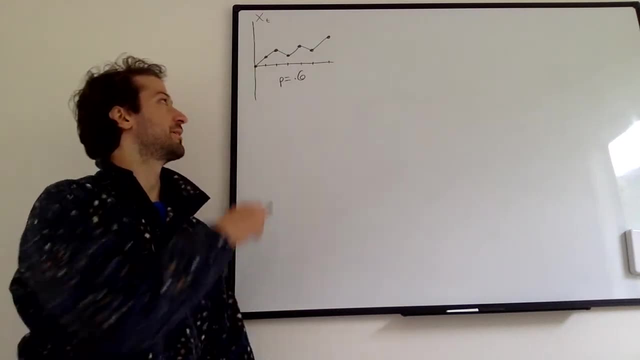 I have some y-axis, you know, instead of any sort of unit time space, which I guess is not really time. but you know, space steps up, steps down, that sort of thing, And you can kind of see the random walk. 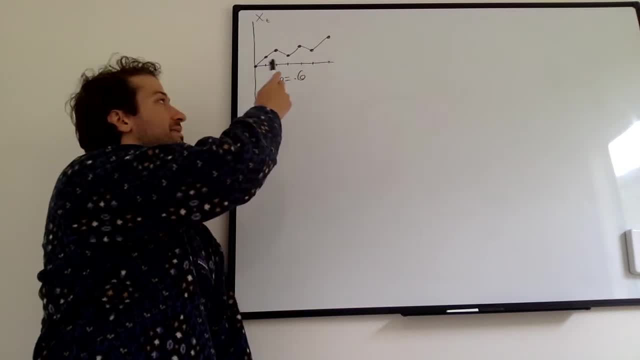 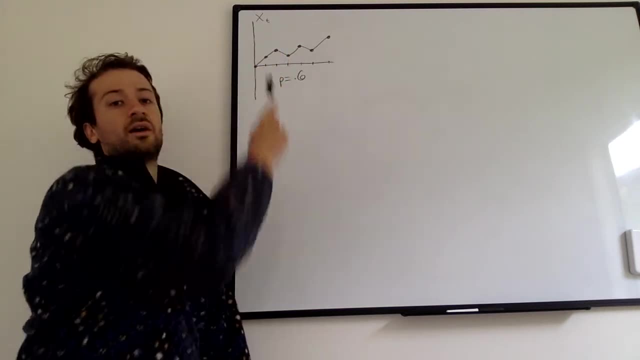 The random walk is the discrete time points labeled on the x-axis or time axis, which means time one time two, time three, and each step we either go up or down at one step. So here it's drifted up a little bit. 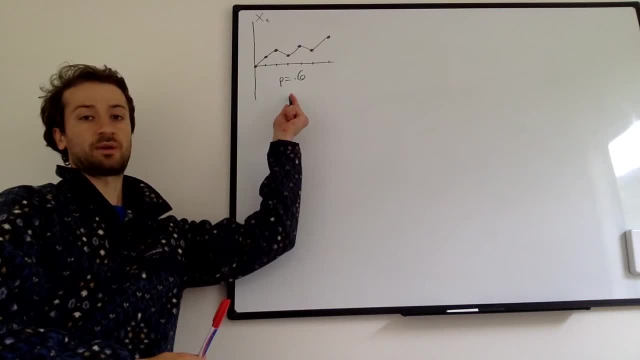 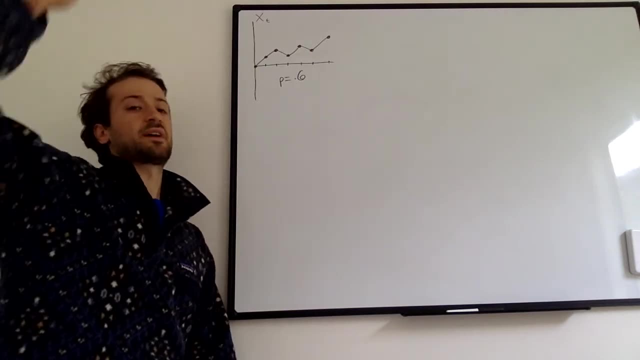 The important parameter for the simple random walk is p, the probability of going up on any one step. In this case, I have p equals 0.6, so you have a 6% chance of going up on any one step, 40% chance of going down. 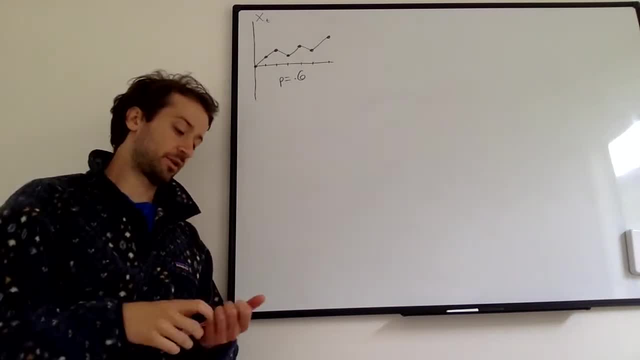 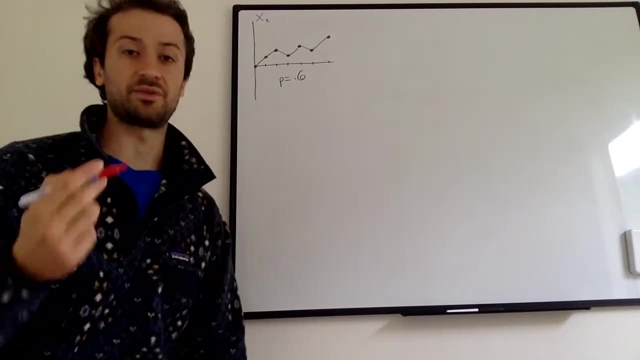 Each step is independent. so in the long run, this is This thing- will kind of drift upwards. So what we're going to be interested in is the probability of hitting a certain value, k. So I kind of just drew it here. 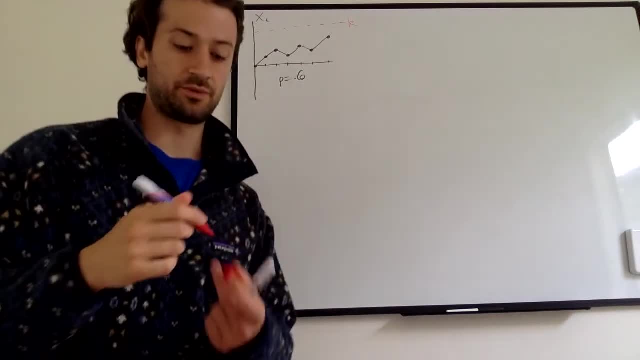 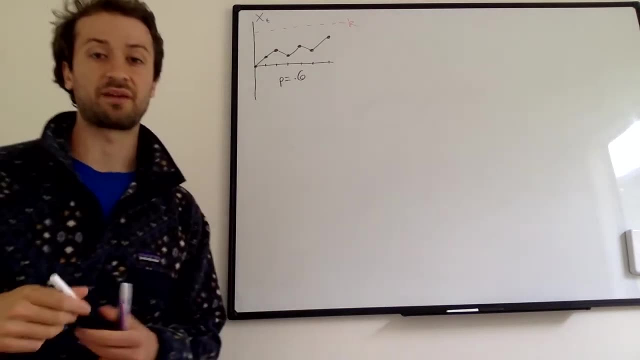 Let's say, you know, I have some value, k maybe k equals 10, k equals 100, k equals 200. And if you let this simple random walk walk around forever, we want to find the probability of ever hitting that value. 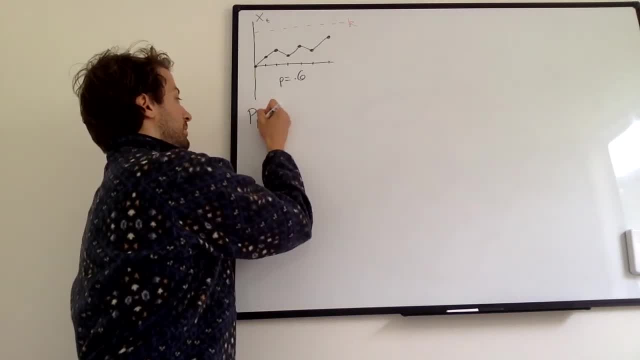 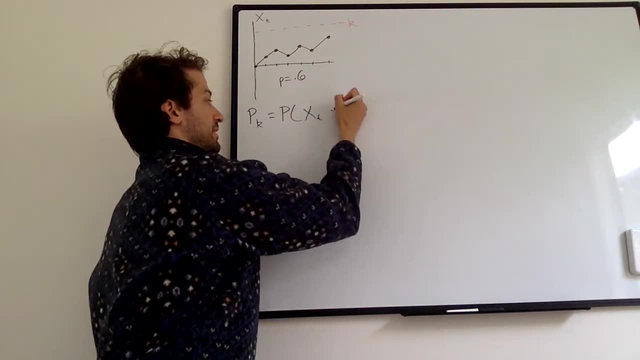 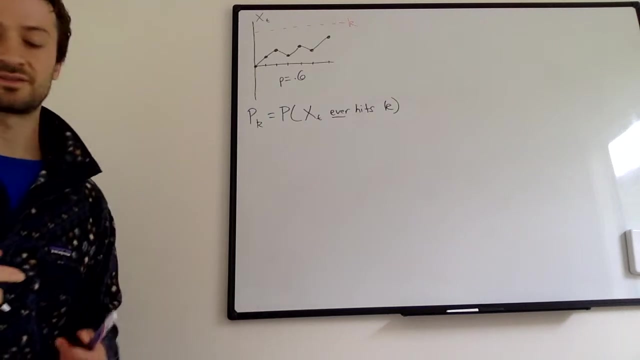 We're going to call that p sub k, p sub k. we're going to say equals Probability, that x sub t, which is our stochastic process, a random walk, x sub t, ever it's. So we could hit it in 20 years, in 30 years, you know which is going to run. 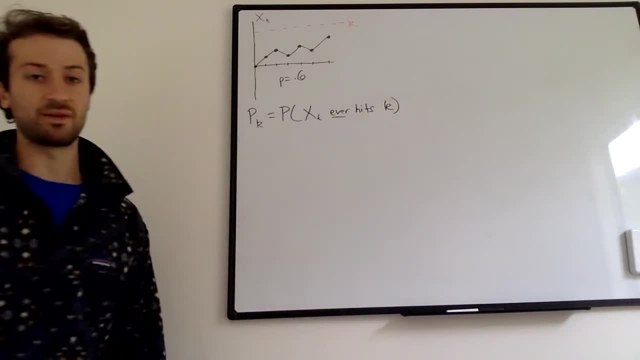 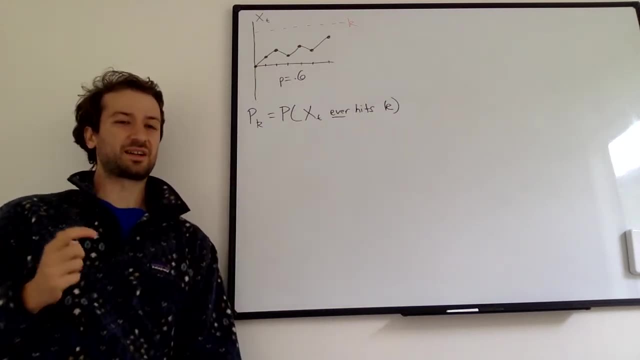 And as soon as it kind of reaches that k value, we've hit k. We want to find the probability that this occurs. So this is interesting to think about, because it's obviously a little bit complex, right? If we allow this stochastic process to run forever, a lot of things can. 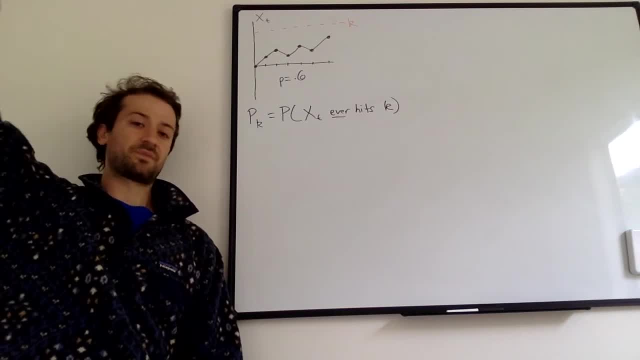 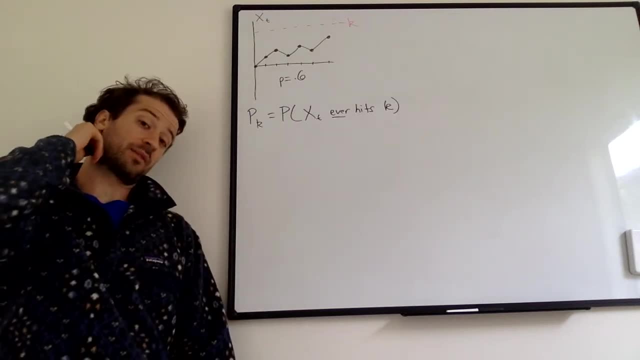 It can happen right. It can go up, it can go down, it can reach the k in a bunch of different ways. It can take however long we need. So this is a little bit complicated to think about, but we can break this down really nicely. 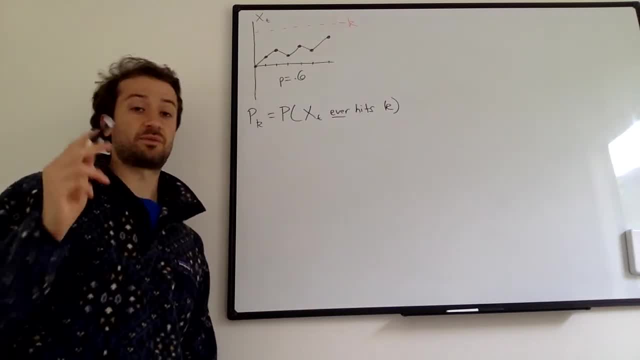 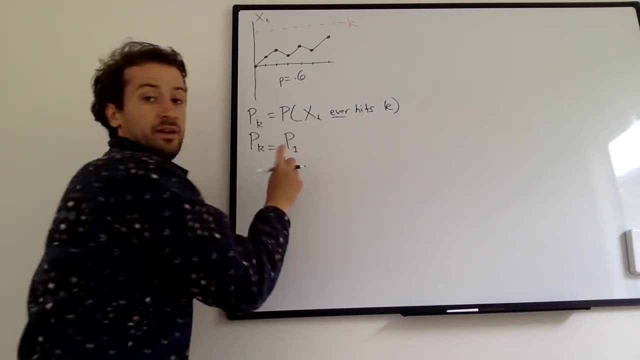 by actually relating this to a much simpler quantity, which we're going to do here. So what's cool is we can say: p sub k equals p sub 1.. p sub 1, right, We're just plugging in 1 for k. 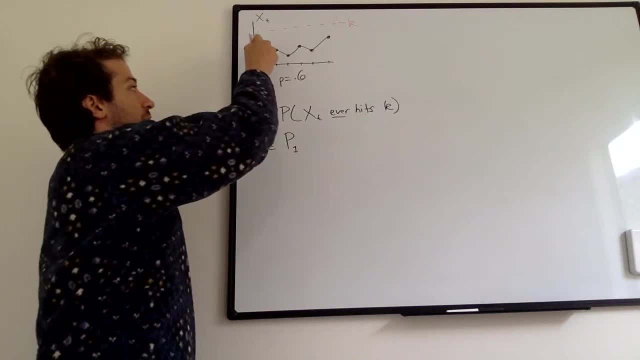 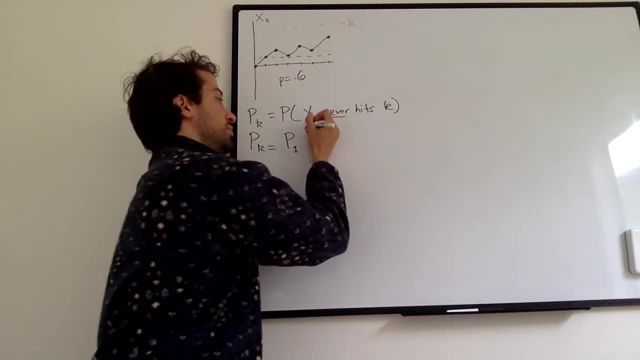 p sub 1 is the probability of hitting 1.. So you know, Here's 1 on our chart. Clearly this random walk hit 1.. The probability of hitting 1 to the power of k. And we can take a second to think about why that makes sense, right. 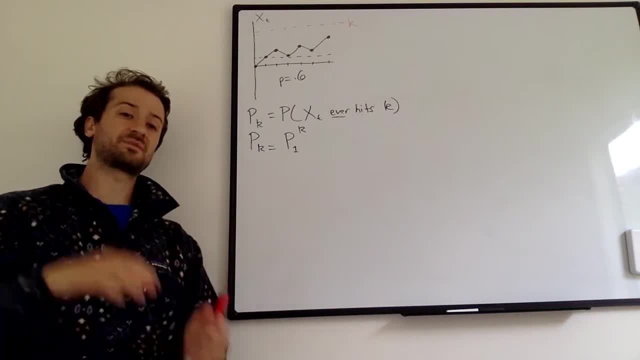 Basically, we want to go up k steps. So going up k steps is the same as going up one step k times, right? So the probability that we make it to one step, the probability that we make it to one step k times, 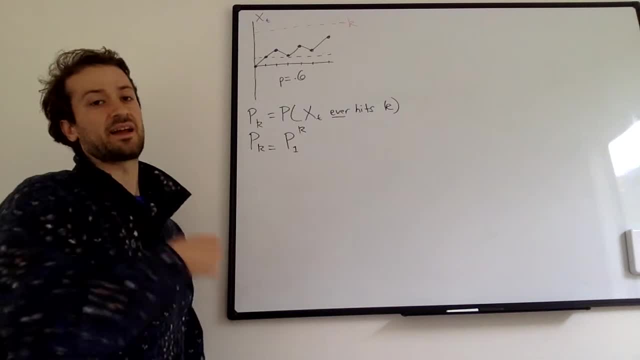 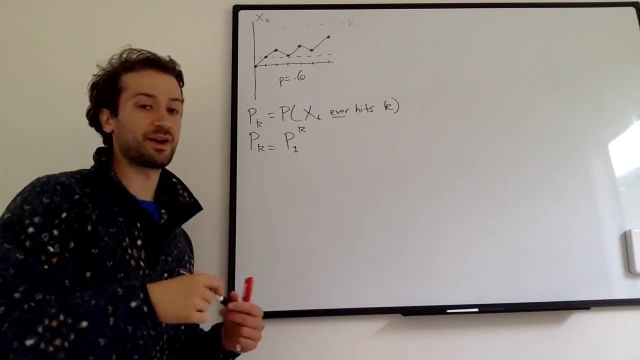 that's the probability that we're going to get to 2k steps. So that's why we raise this to k. Each step is independent, so we can multiply the probabilities, We get this cool result, And p sub 1,, as you can probably guess, is way easier to find than p sub k. 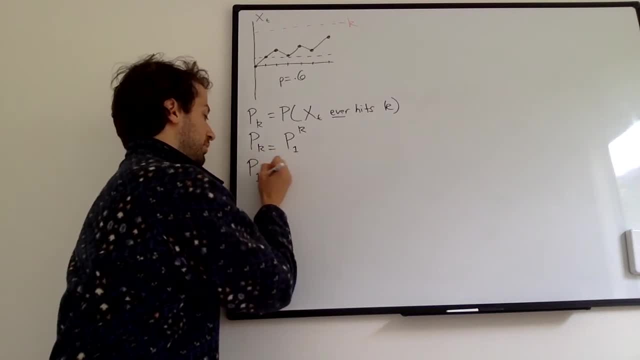 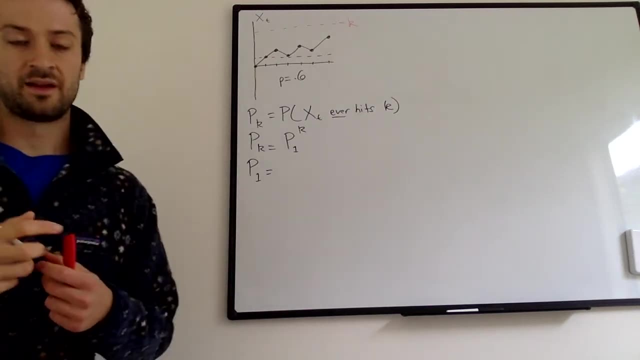 which is exactly what we're going to do. So to find p sub 1, we're going to use something called first step conditioning, Conditioning on the first step, law of total probability. Basically, we're going to think about Conditioned on the first step of the simple random walk. 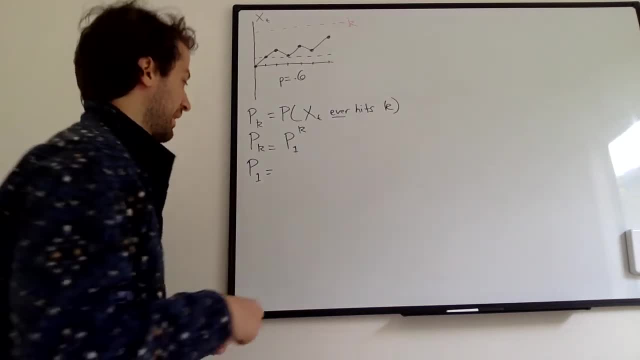 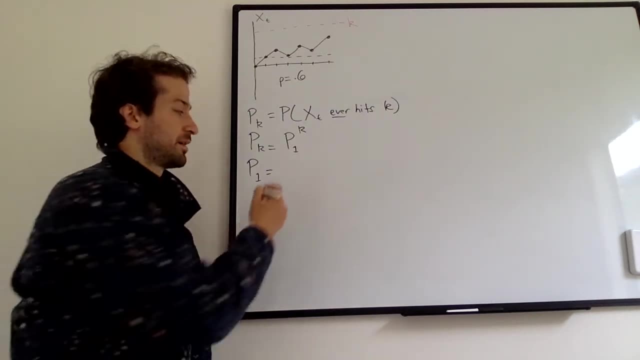 what's the probability that we ever hit the value on? Okay, And we can break it down into two cases: The simple random walk- It goes up on the first step or down on the first step. So you know we have probability p right that we go up on the first step. 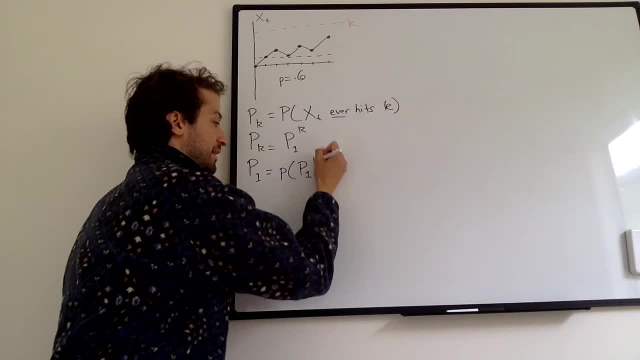 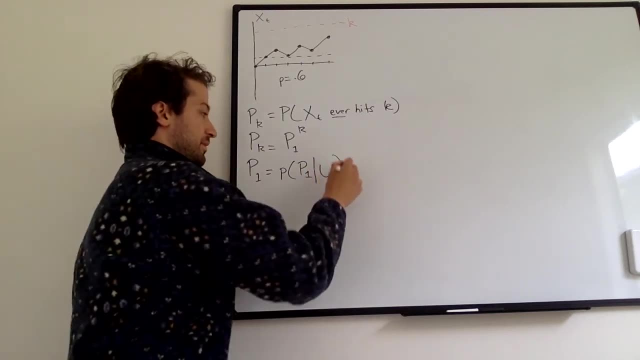 And then we're going to multiply that by p sub 1, given that we went up on the first step. So I'm just using u to indicate the event that we went up on the first step. So this is a little confusing. I have p. 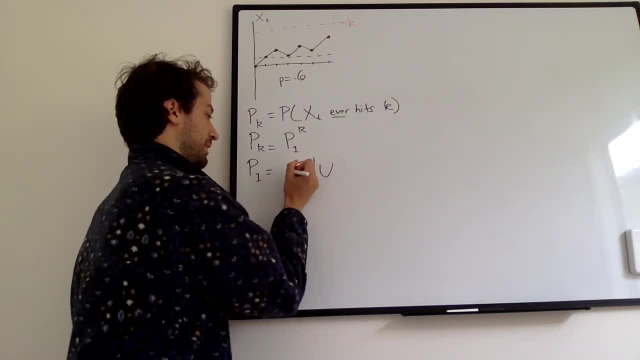 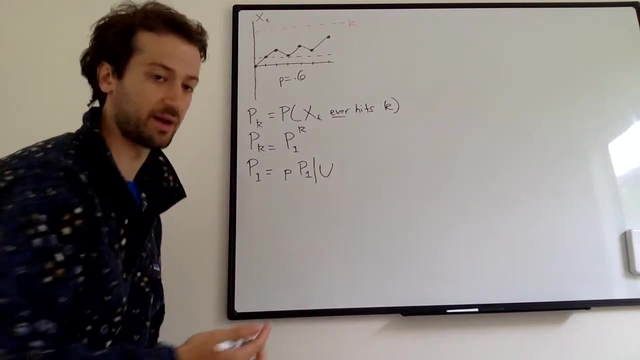 So it kind of looks like I'm doing probability x, Let's just do this p. So the probability that we went up on the first step times the new probability that we're going to hit 1, given that we went up on the first step, plus q. 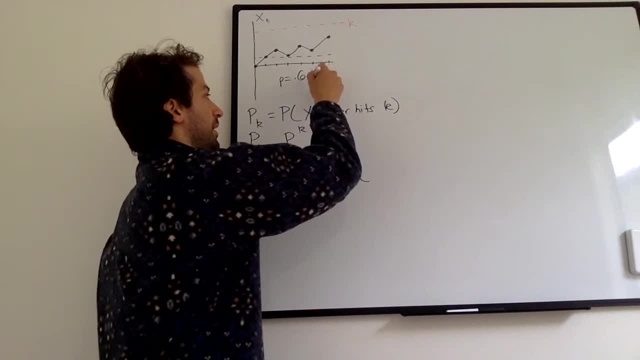 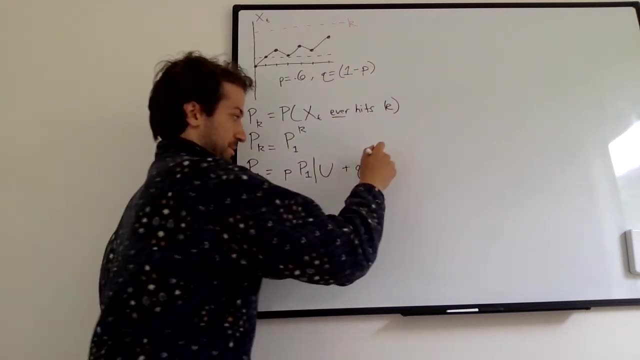 q is just 1 minus p. Instead of writing 1 minus p, we just use q. I'll actually write that here: q equals 1 minus p Plus q times new probability of hitting the first step, given that we went down on the first step. 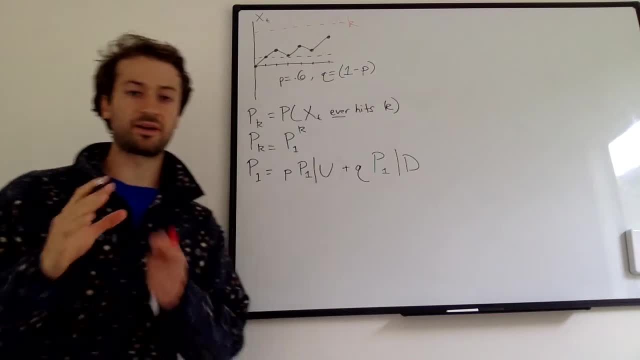 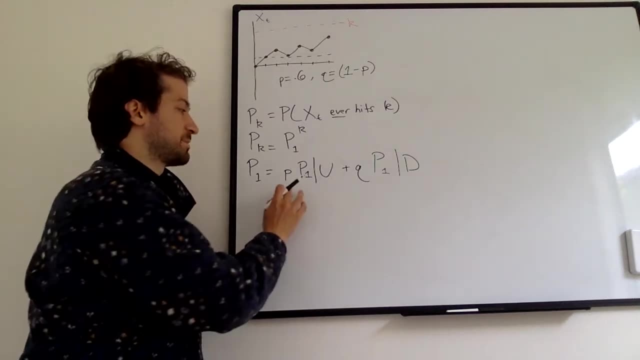 Okay. So law of total probability: Break the world into different cases. You know, weight the cases by the probability that those worlds occur. So we look at each of these terms. p and q are constants. They're given based on the problem. 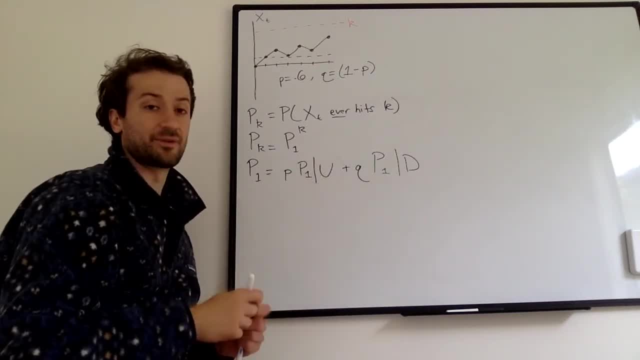 Probability of hitting 1, given that we went up on the first step. Well, that's just 1, right, Because we went up, We hit 1.. We're done. p sub 1 is now 1.. We went up. 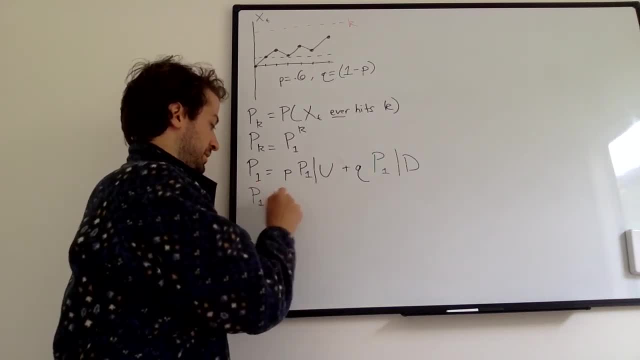 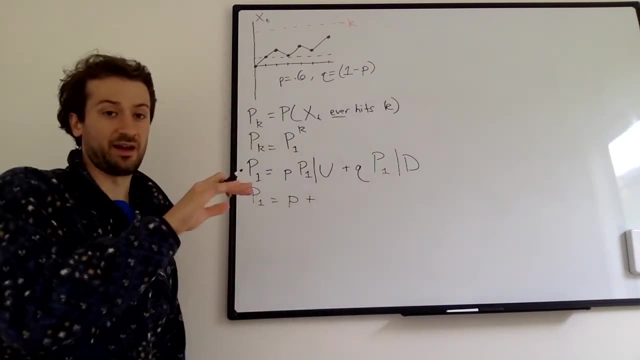 It's all good, So that term just becomes p. This term is a little bit trickier: p sub 1, given that we went down, So we're actually a negative 1. now What's the probability that we hit 1?? 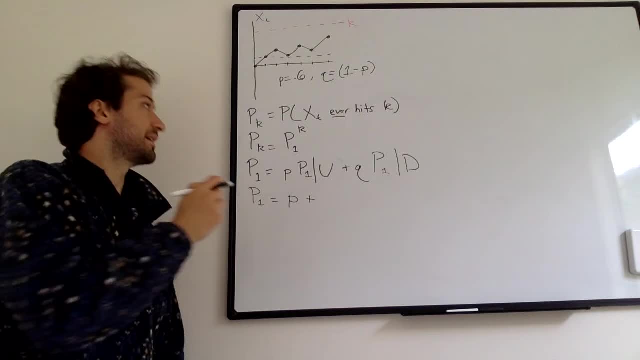 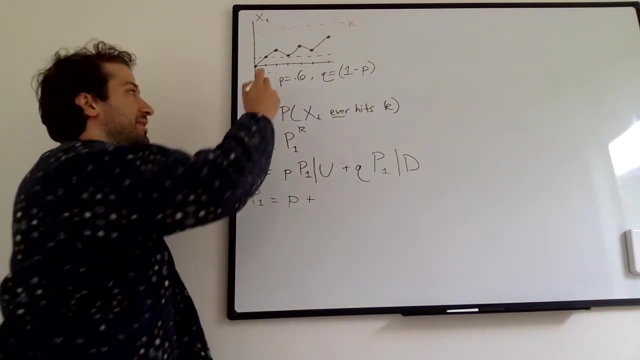 Well, we can actually, Basically, we think of if we're at negative 1 and we want to hit 1, that's the same as starting from 0 and hitting 2, right, So we go from negative 1 to 1 to 2 eventually. 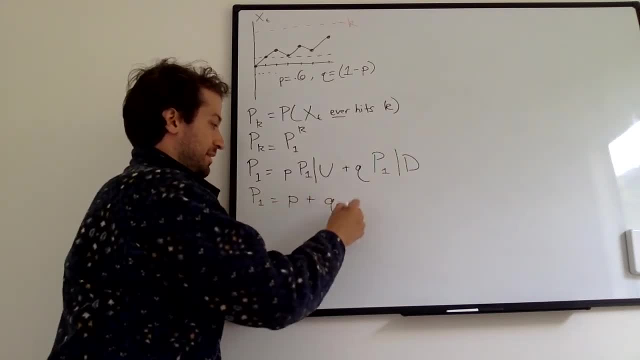 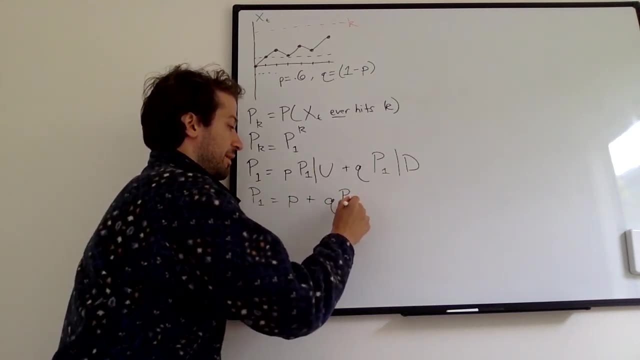 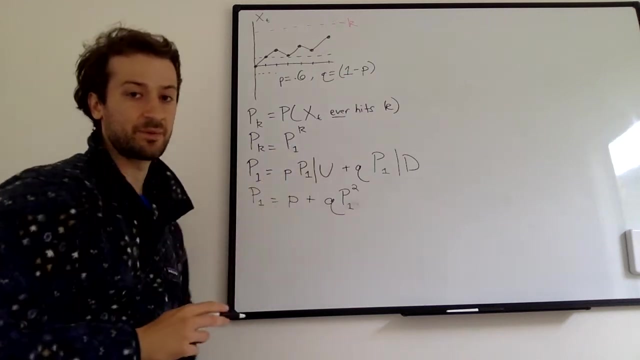 So that's the same as hitting 2, which is q times p sub 2, right. But instead of writing p sub 2, we can just say p sub 1 squared right, Basically going up twice, and we're using this formula: p sub 2 equals p sub 1 squared right. 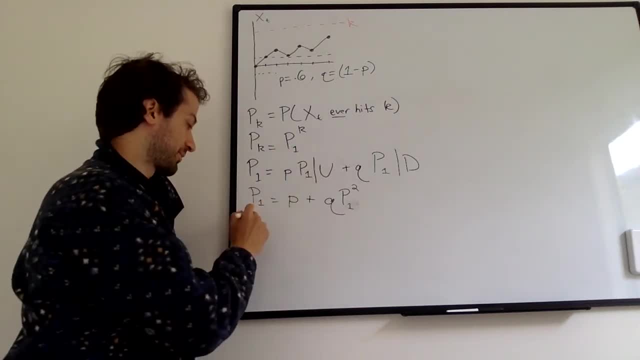 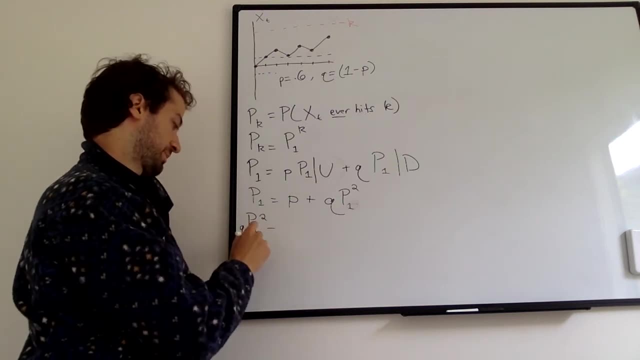 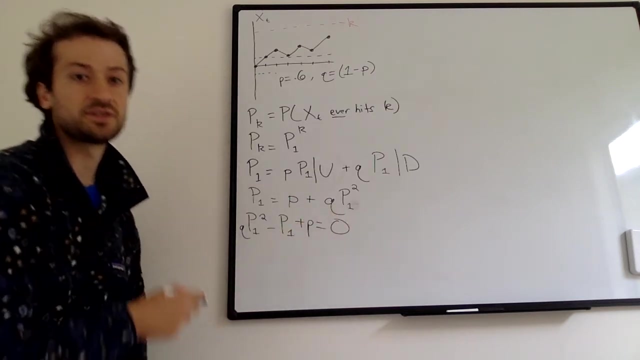 So we have this nice term Which is totally in terms of p sub 1.. And I can move everything to one side, So q, p sub 1 squared minus p sub 1 plus p equals 0.. That looks like a quadratic equation. 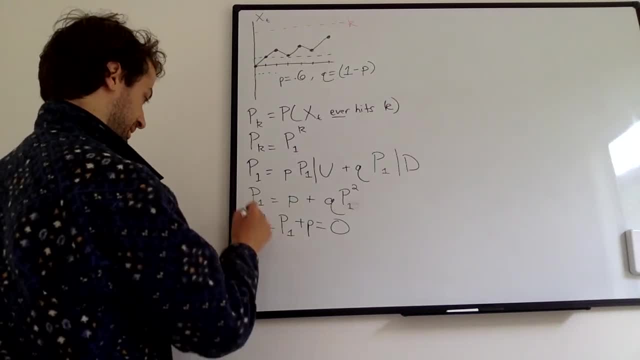 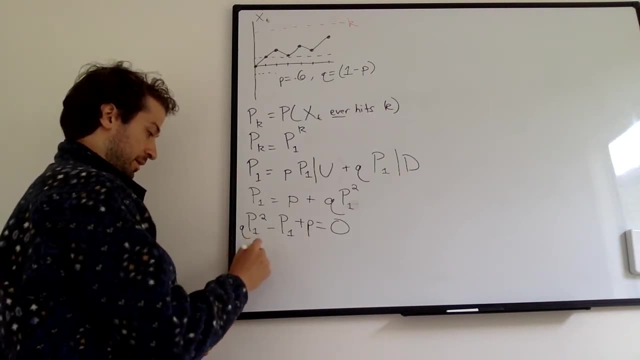 We can use a quadratic formula to solve it right. So we have minus b. Remember q equals a Negative, 1 is b, p is c. So we have minus b. So 1 plus or minus the square root of b. 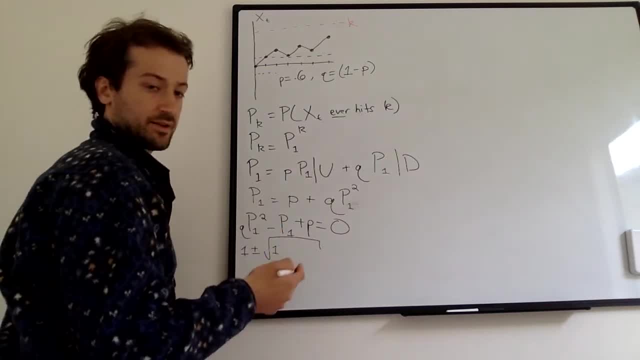 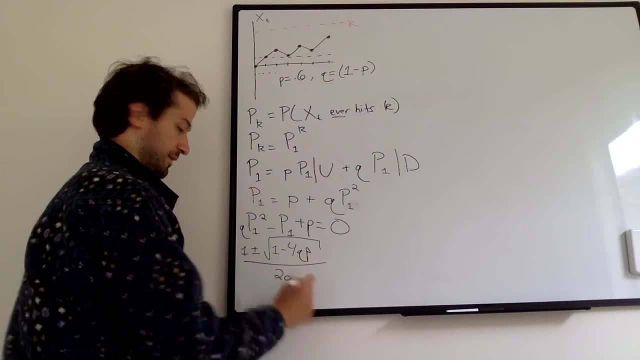 So that's 1. b is negative, 1. Minus 4ac, minus 4qp, All over 2a. Okay so that's our quadratic formula, And this looks like a little bit weird to solve because it's square root of 1 minus 4qp. 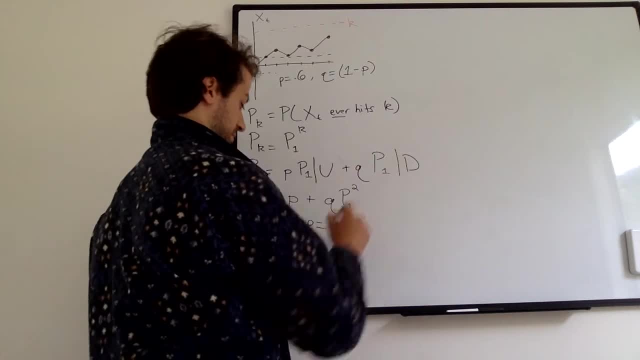 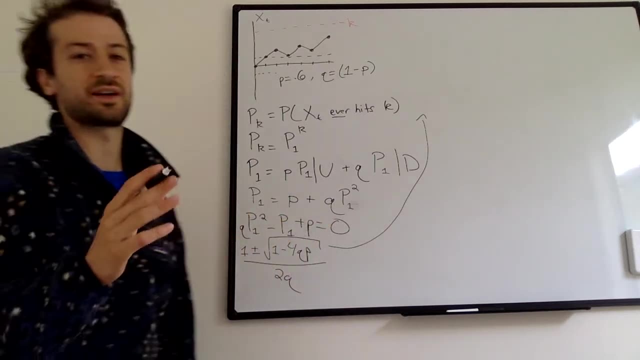 But we actually have a trick to solve that. So we're going to go over here Kind of work that out. So we're going to use a trick here. It's kind of a weird trick. You might not think of it From the start. 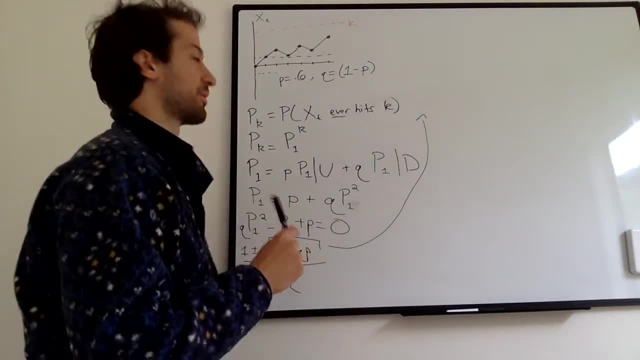 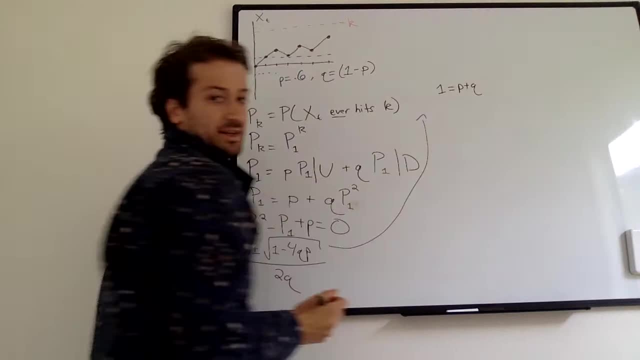 But it's a useful trick to kind of break this weird square root thing down. So we know that 1 equals p plus q, And that's because p is the probability that the thing goes up. The random walk goes up, q is the probability it goes down. 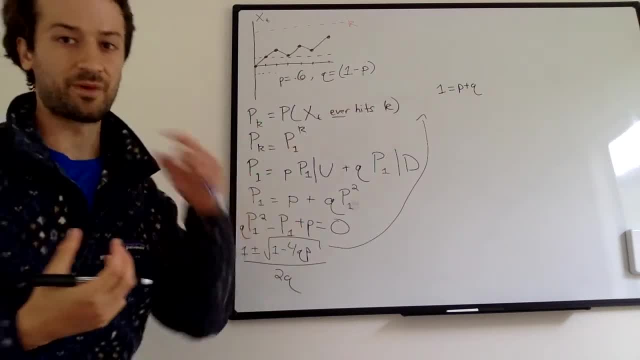 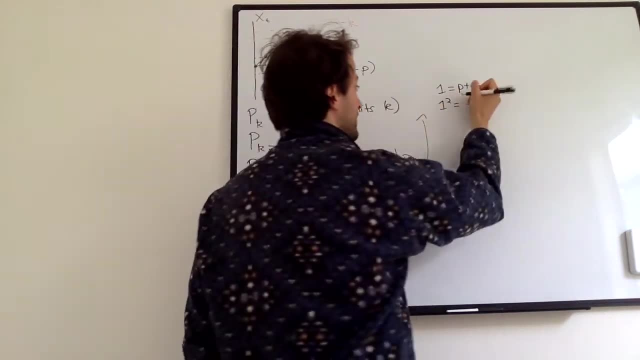 More simply, p plus 1 minus p is going to be 1.. So we know this is true. We square both sides, Square both sides, We get 1 squared which is 1.. 1 squared equals p plus q squared. 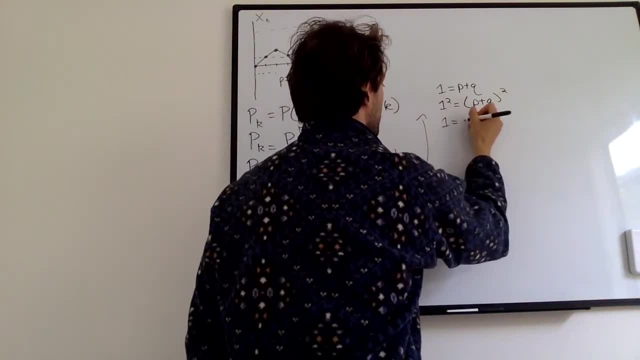 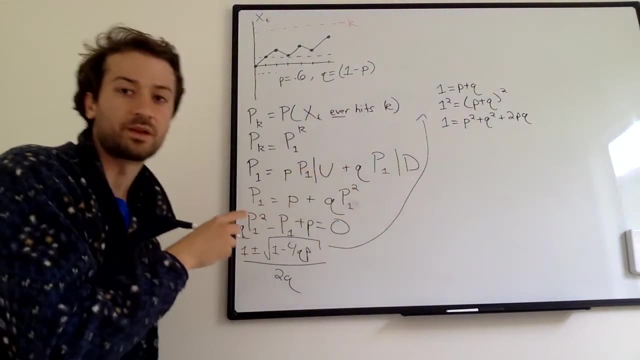 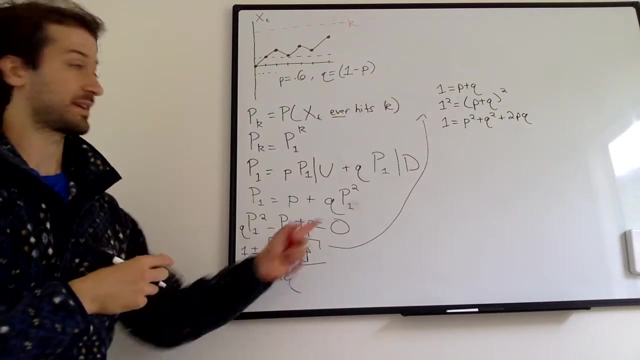 We can expand the terms, So 1 squared becomes 1.. Right, I have this 1 plus, you know, p squared plus q squared, And now I want to make this term look something like this term. So I'm going to subtract. 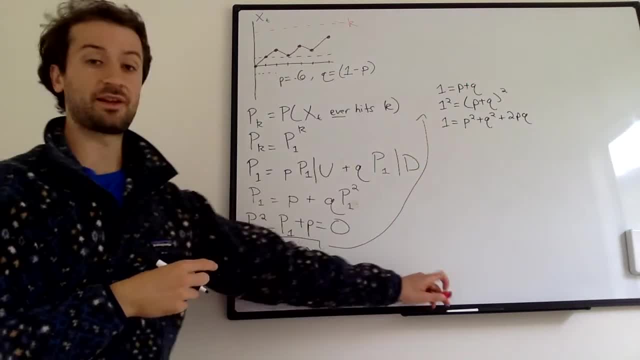 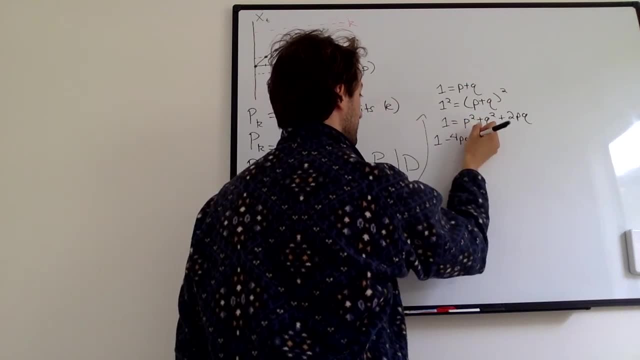 I already have 1 on this side. I'm going to subtract 4pq from both sides Right. So subtract 4pq from both sides, You get 1 minus 4pq. 4pq equals p squared minus 2pq. 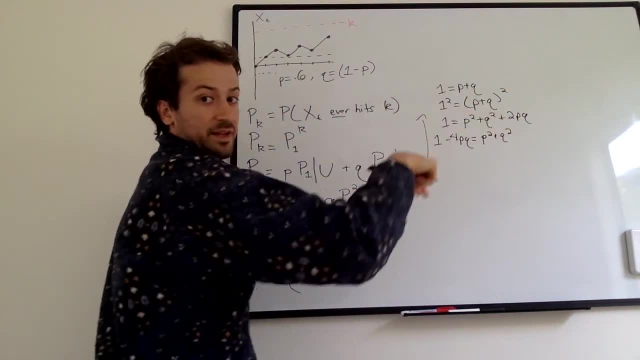 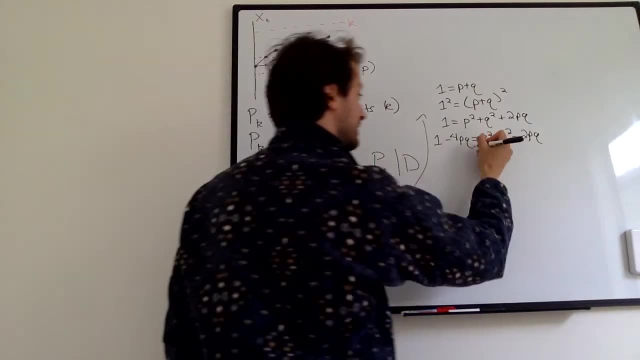 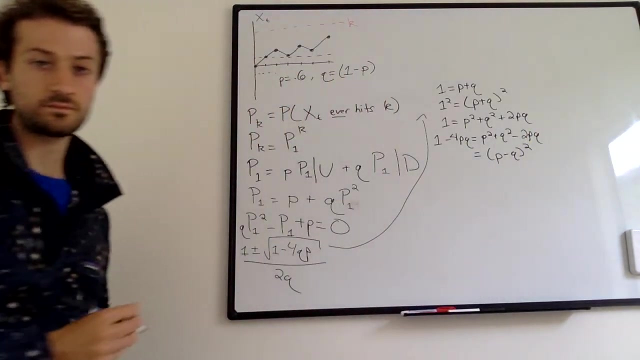 Now we had 2pq originally on this side. Subtracting 4pq, we get minus 2pq- Awesome, Minus 2pq. This right-hand side simplifies: 2p minus 2p squared Awesome. 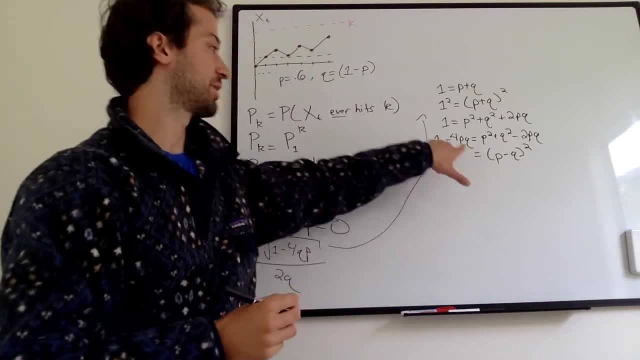 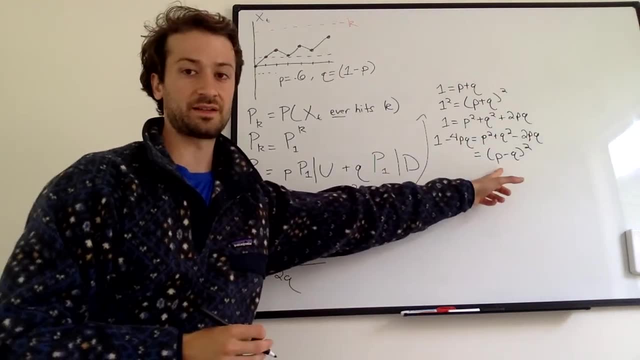 p minus q squared. This is way easier to plug. You know. you've shown that 1 minus 4pq equals p minus q squared. Way easier to plug into this quadratic formula. So we're taking this formula, plugging it into here. 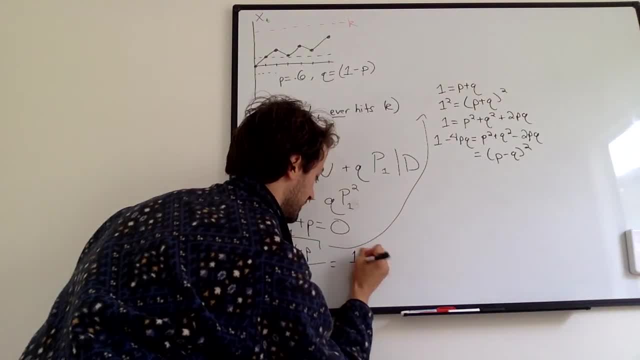 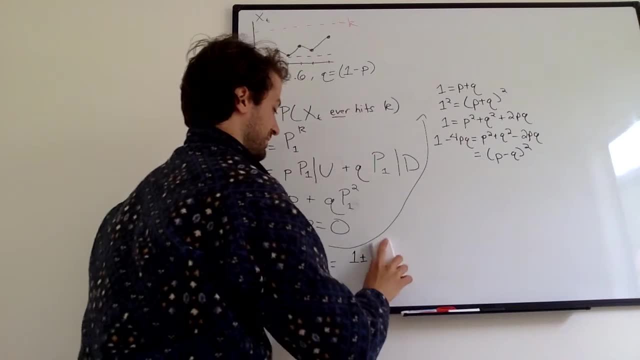 So we'll just do the whole thing now: 1 plus or minus square root. Square root of p minus q. squared is just pq. There's, you know, technically we're taking a square root of something that could be negative, But you're going to see in our answer that we adjust for that. 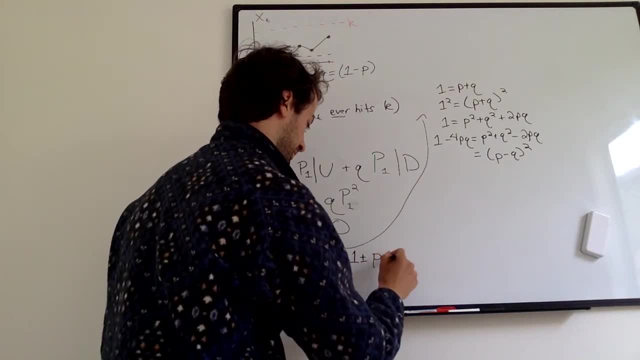 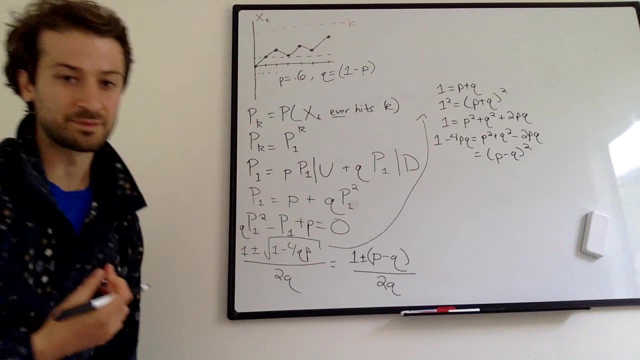 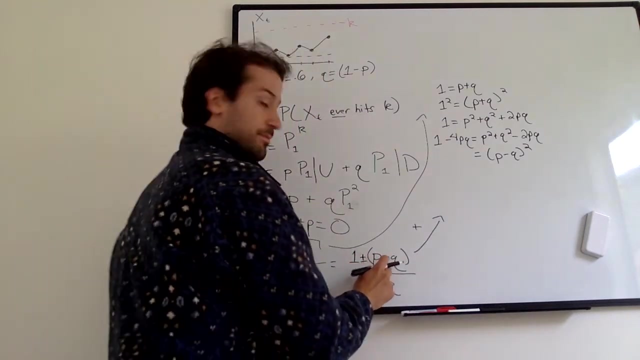 The square root of p minus q. squared is just p minus q, All over 2q, And this is way easier to work with. This is just arithmetic at this point, So let's do the plus case, So 1 plus p minus q. 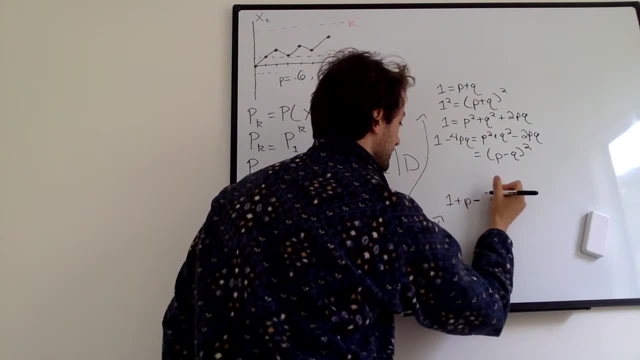 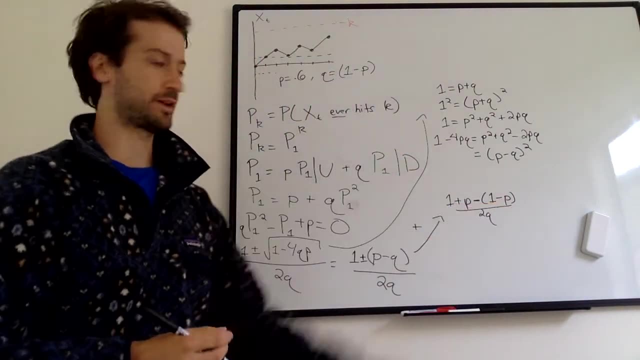 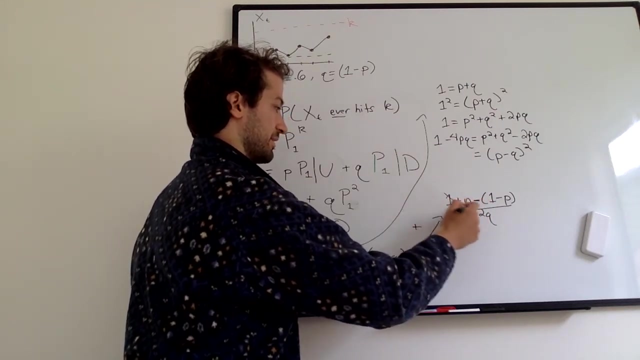 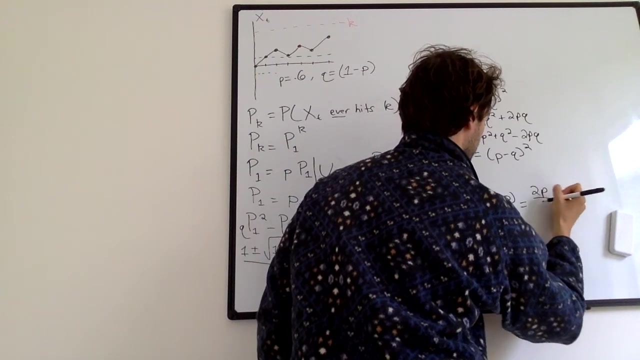 So 1 plus p minus 1 minus p, All over 2q. I plug back in 1 minus p for q here. So I have 1 plus a minus 1 and then p. So the 1's cancel And then p minus a minus p get 2p equals 2p over 2q. 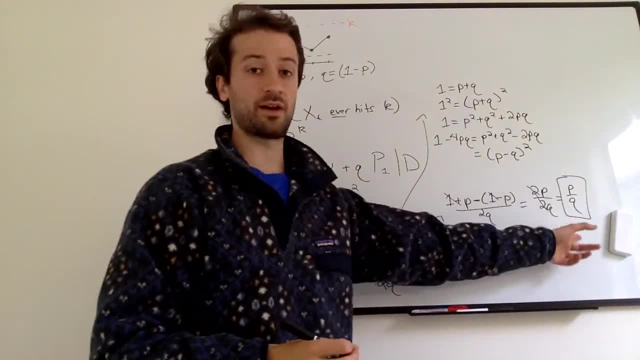 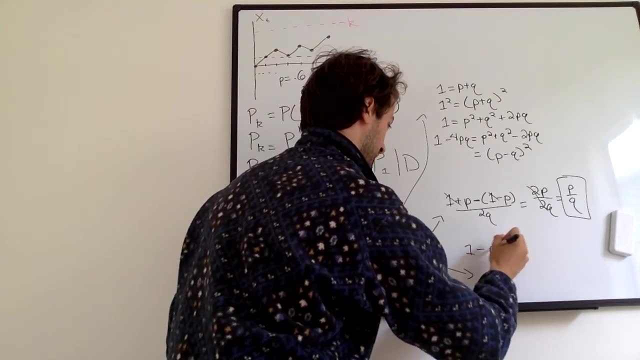 Keep those straight: P over q is one solution. And now, if we do the minus, we get 1 minus p, plus 1 minus p, 0 over 2q, 1. Minus 1. Minus 2.. 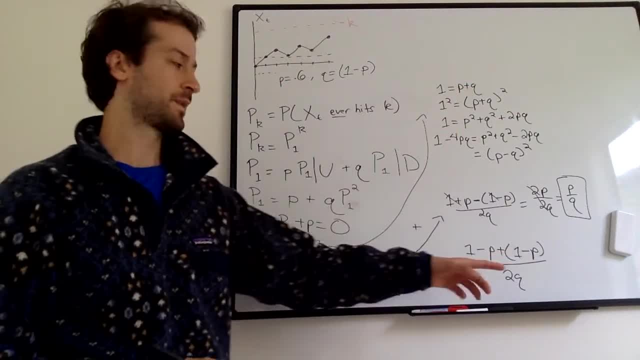 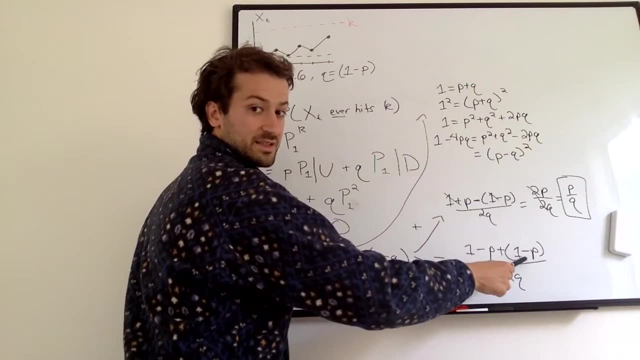 So this is the minus case: 1 minus p plus q. I see 1 minus p plus 1 minus p. 1 minus p is q. This 1 minus p is q. I have 2q on top over 2q. 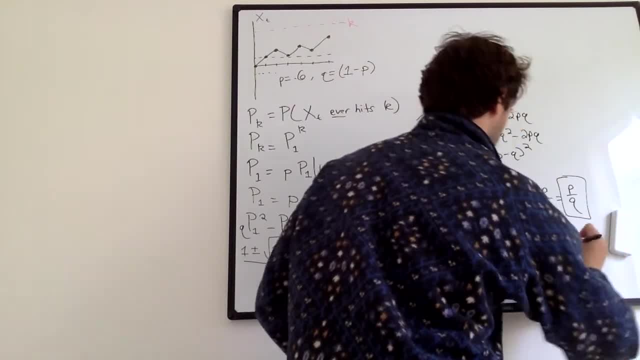 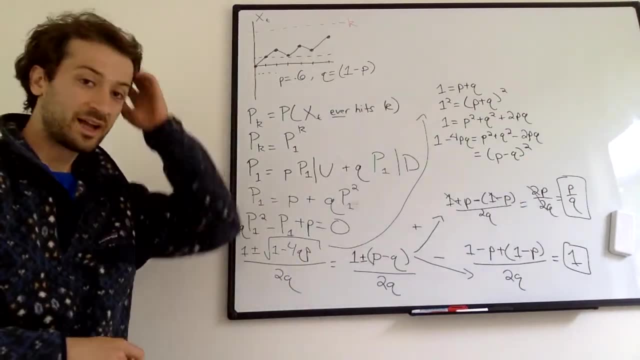 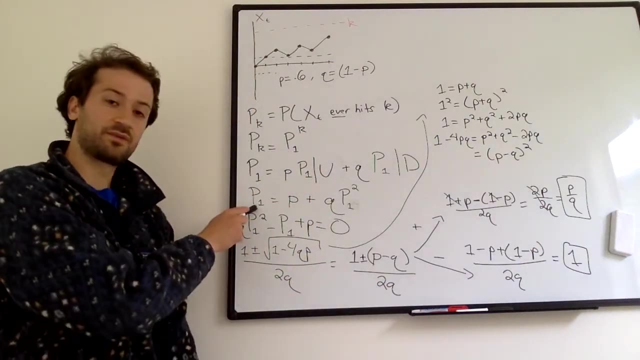 That's equal to 1.. Awesome, So we have these two solutions. How do we know which one to use where? Well, if you look at this solution, p over q, right. This whole. what we're solving for is p sub 1, right. 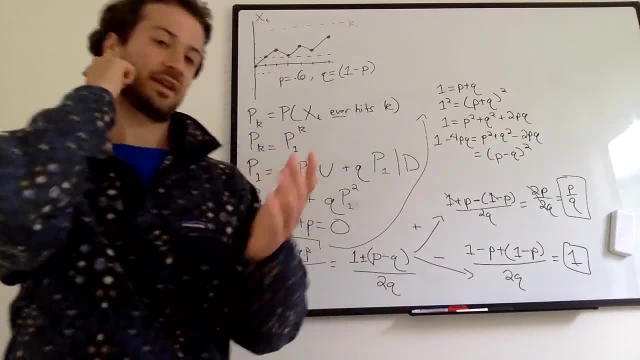 So we're solving for a probability. The probability must be between 0 and 1.. That's one of the axioms of probability. If p is greater than q, then this is going to be greater than 1.. So this will not work. 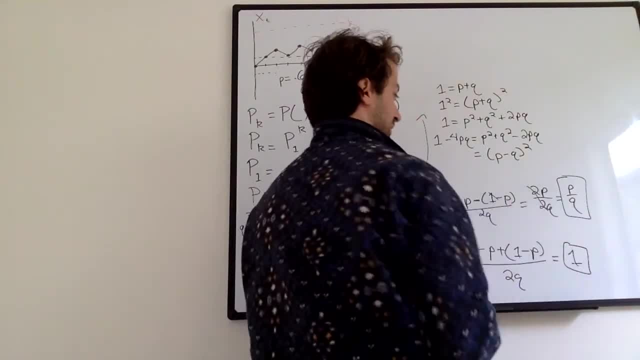 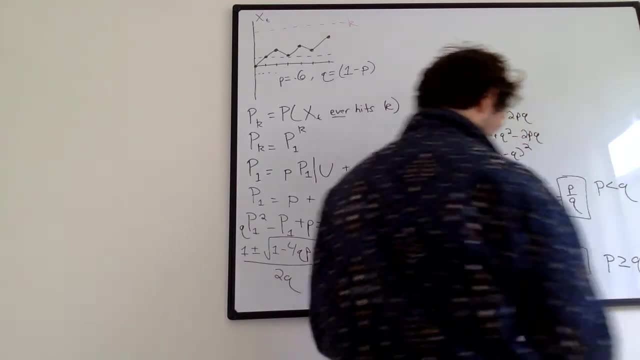 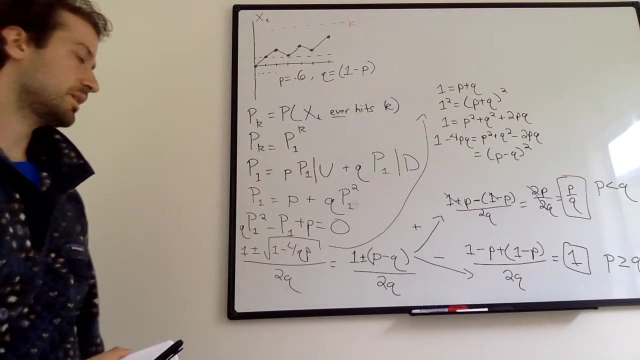 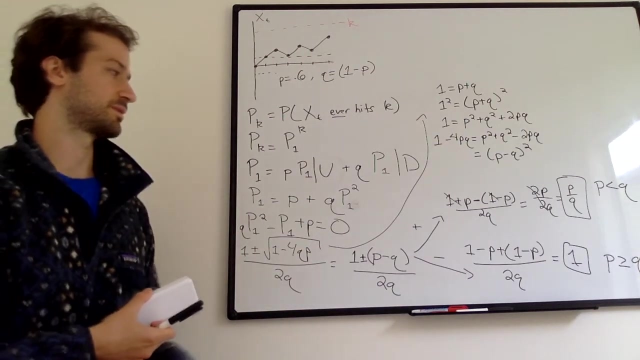 So in that case we're going to use this solution So we can say p over q, And that's why, when we took the square root, this thing kind of worked. We don't really have to worry about in that case, because we're just going to use 1 in certain parts of the solution. 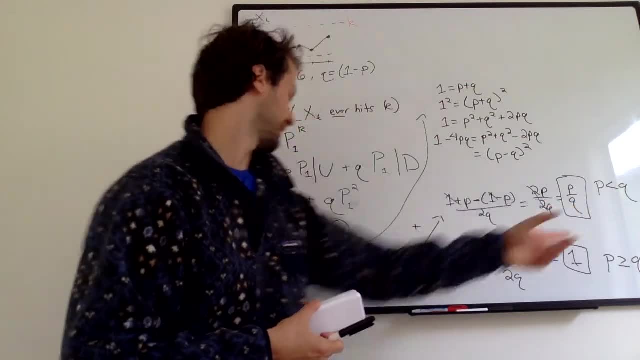 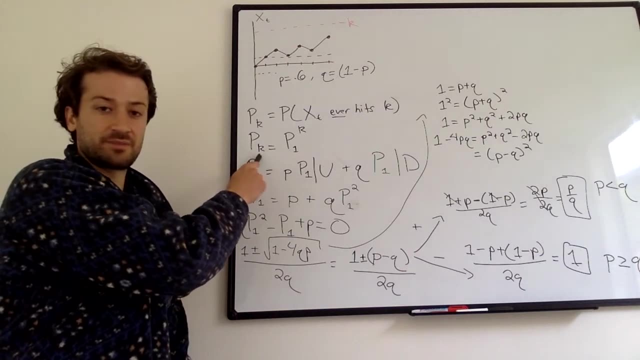 So let's take a second and look at this. This is kind of our result, And we solve this for p sub 1, or the probability of ever hitting step 1.. And remember, we did this fancy thing where we said probability of hitting k is just p sub 1 to the k. 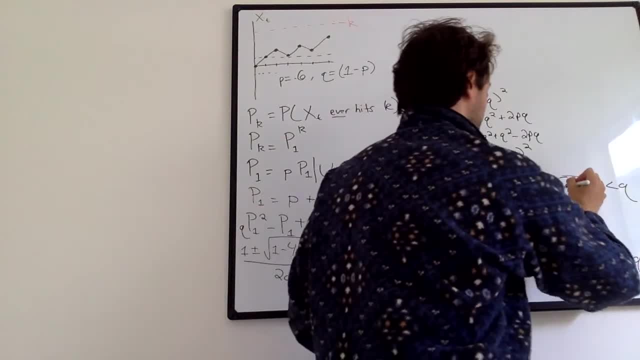 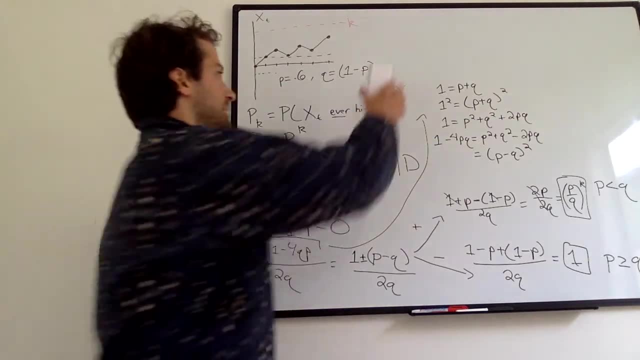 So if we wanted to solve this for k, all we do is raise this to the power of k Right And 1 to the power, So the power of k is still just 1.. Okay, so now we have really simply the probability for any random walk. 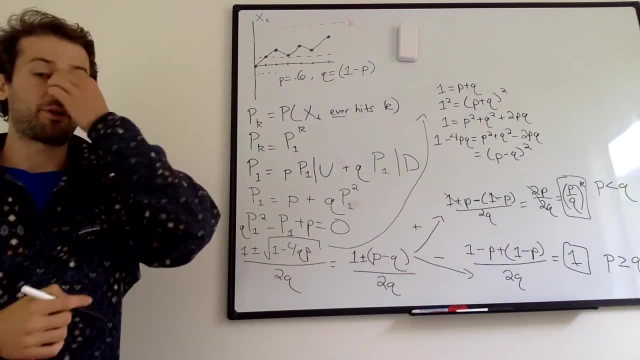 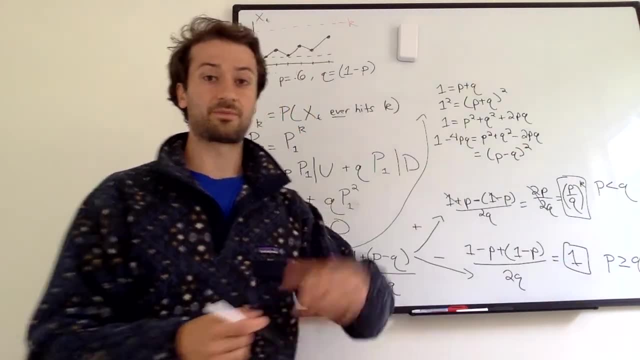 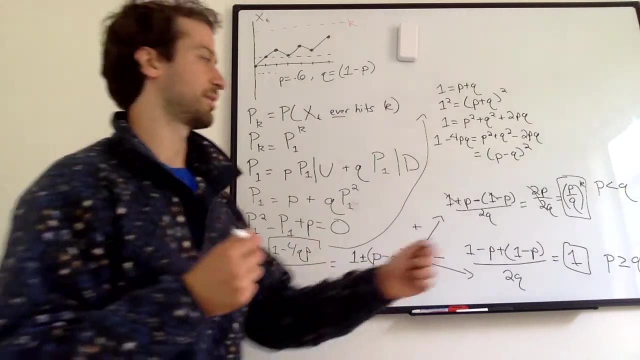 the probability of hitting a certain value, k is just p over q to the power of k. Okay, when p is less than q, and the probability of hitting k when p is greater than or equal to q is 1.. And I was just stuttering because I realized we could make this simpler. 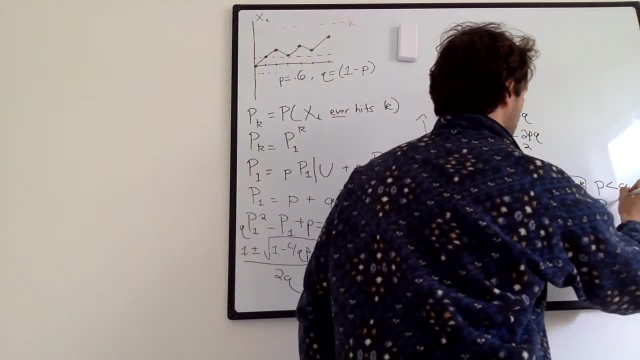 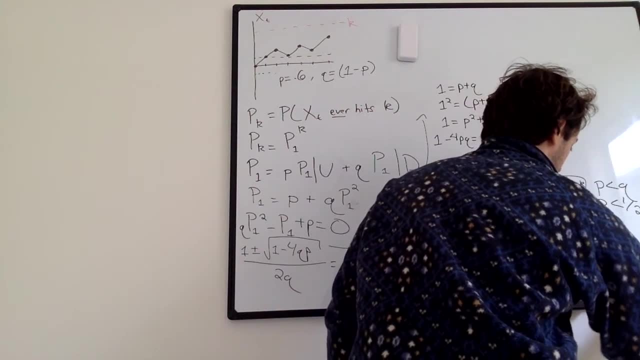 p is going to be less than q when p is less than 1 half. Okay, p is going to be greater than or equal to q when it's greater than 1 half, Greater than or equal to 1 half. Right, So we can start to develop some intuition around this, right? 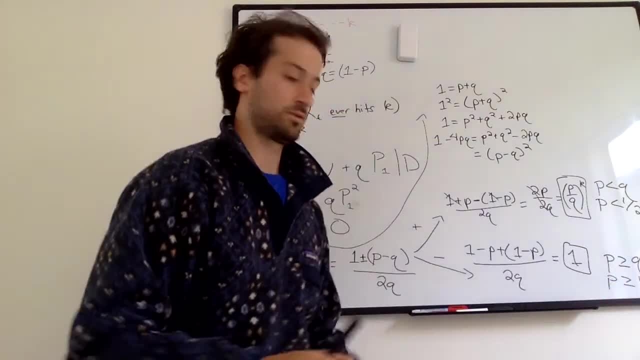 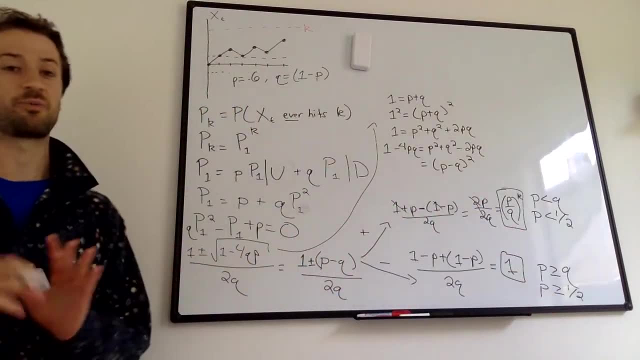 When p is greater than or equal to 1 half- right, Oops, sorry, you're out of screen. When p is greater than or equal to 1 half, this is saying that we have 100% probability of hitting any value for k. 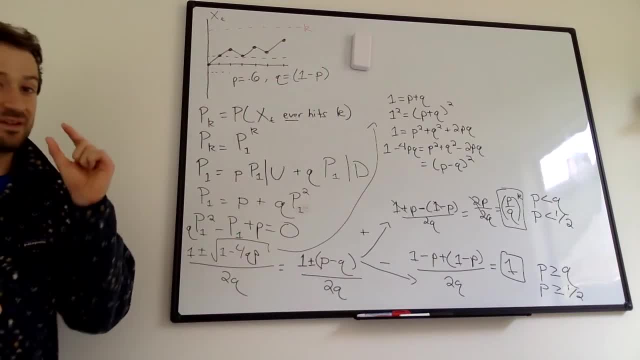 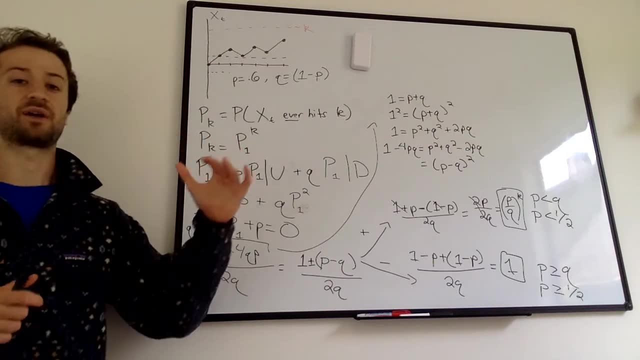 Right, No matter how high k is, and no matter if p is a little bit over 1 half or exactly 1 half, this thing will drift upwards or just drift around Until it hits that value. And it will certainly at infinite time hit, you know, any value k. 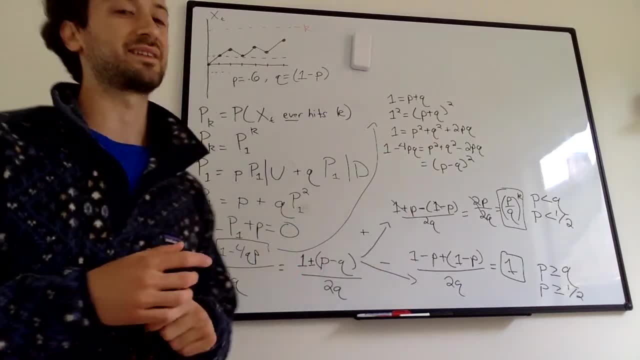 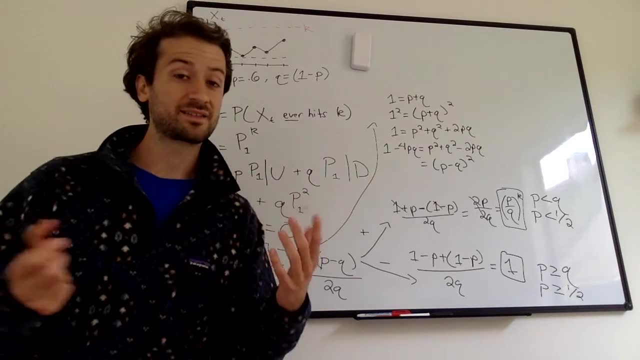 Which kind of makes sense, Because if you let something run forever and it's drifting upwards, it's going to get pretty high. This value is saying that if p is less than 1 half, right, You can imagine, if p is like a lot less than 1 half, we could start off going down and maybe make a little bit of progress back. 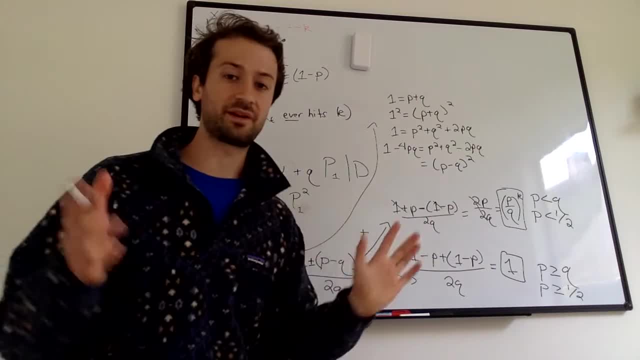 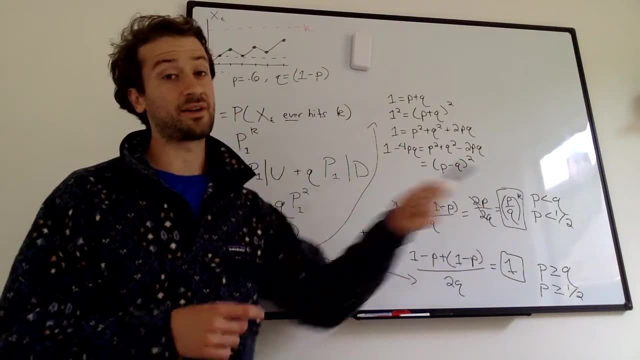 But eventually we're going to go down a lot and we're just going to be so far out of range that we never can hit k. And this is saying that you can see, the smaller that p gets, p will be small, q will be large and this value will get smaller. 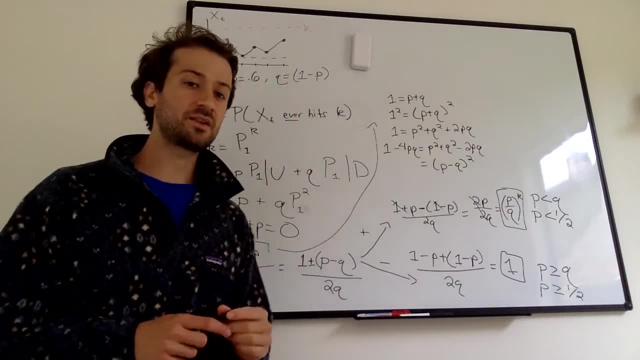 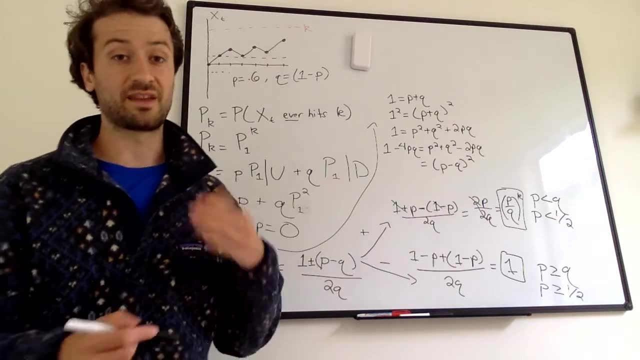 So the lower probability of going up on any one step is going to decrease your probability of ever hitting k, And also we have. you know this power is raised to the k. p divided by q is less than 1, in this case, 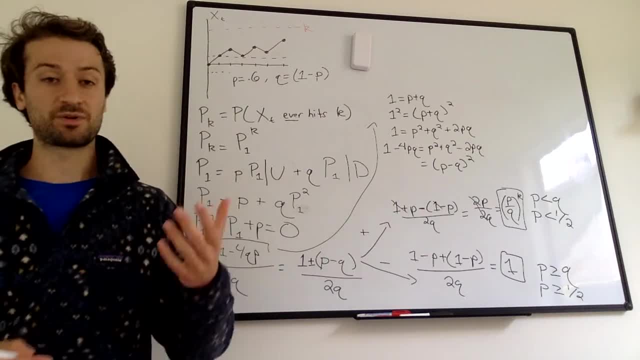 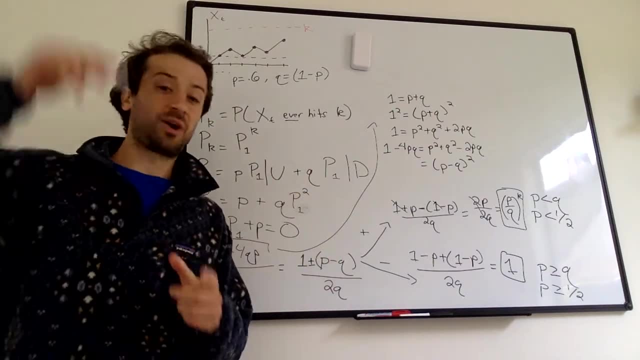 When we raise something less than 1 to the k, it's going to get smaller and smaller as k gets bigger. So you know, k equals 10 is going to be lower than k equals 100, which makes sense, Like it's going to be harder to hit. it's going to be a lower probability of hitting 100 than it is. 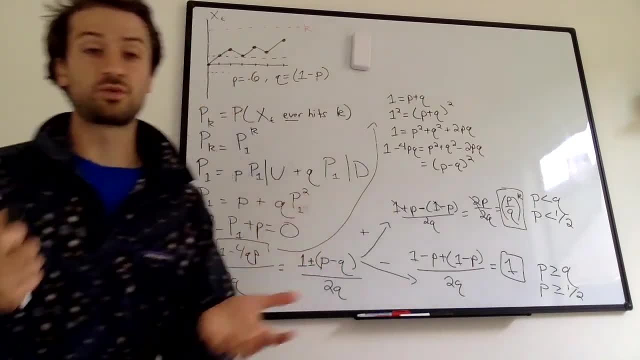 of hitting 10.. So you know, this is kind of intuitive. But what's cool is that this is a very, very like open-ended problem. It seems like very complicated, but it can be reduced in this really simple way. 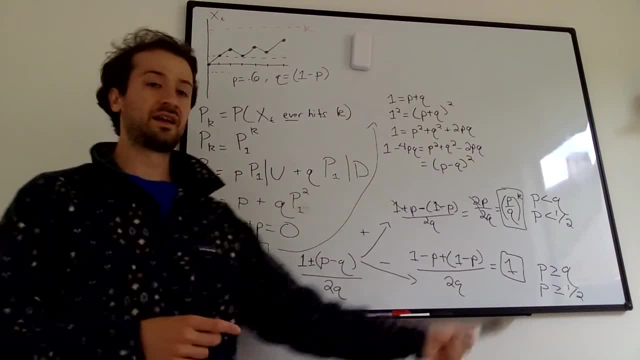 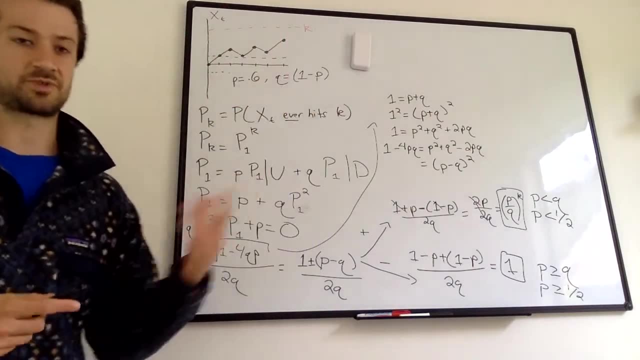 kind of with this step of considering one step at a time, And we get this really, this really neat answer And we're looking at the probability of hitting a positive k. You can absolutely flip this symmetrically and think about hitting a negative k. 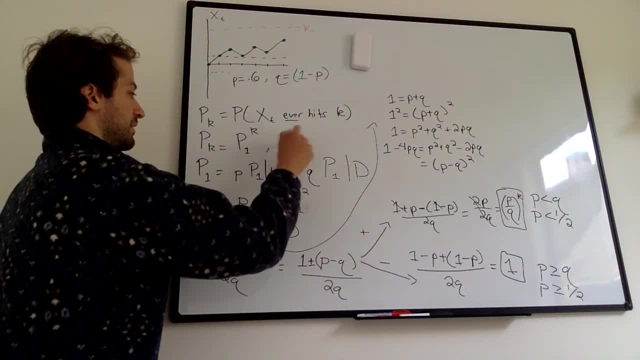 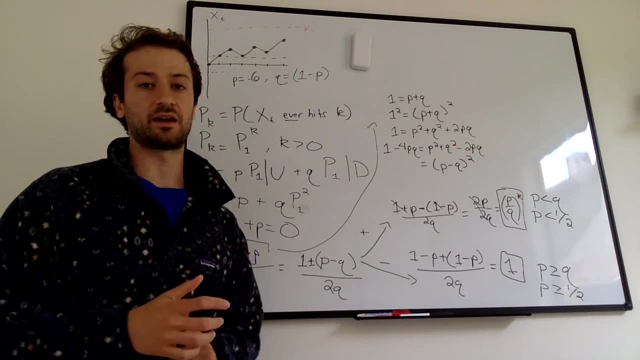 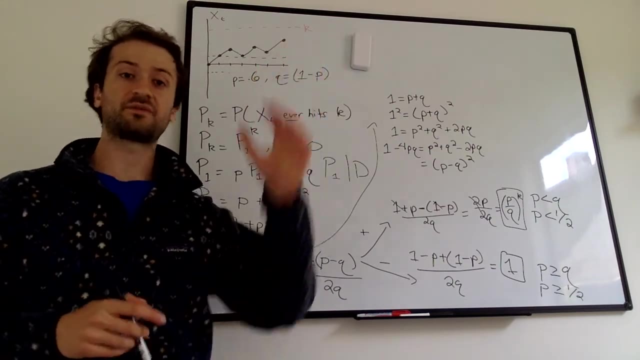 I should. I should clarify: this is for k is greater than 0.. You can flip this. It's totally symmetric if you want to think about the probability of hitting a negative k. So hopefully that helped And we'll be back soon in terms of we'll be thinking instead of the probability of hitting a certain value. the expected amount of time to hit a certain value. So stay tuned. 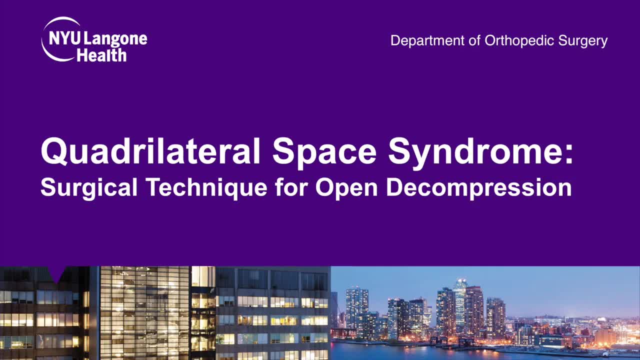 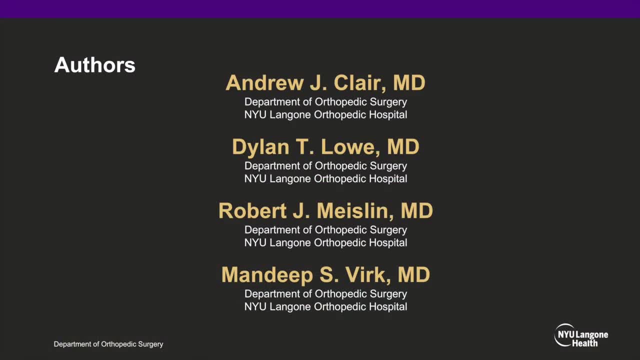 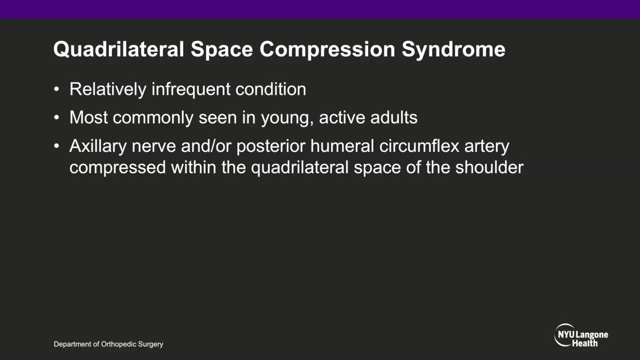 The following video demonstrates a surgical technique and case presentation for the decompression of the posterior branch of the axillary nerve within the quadrilateral space. Quadrilateral space compression syndrome is a relatively infrequent condition experienced by young active adults, in which the axillary nerve and or the posterior humeral circumflex artery 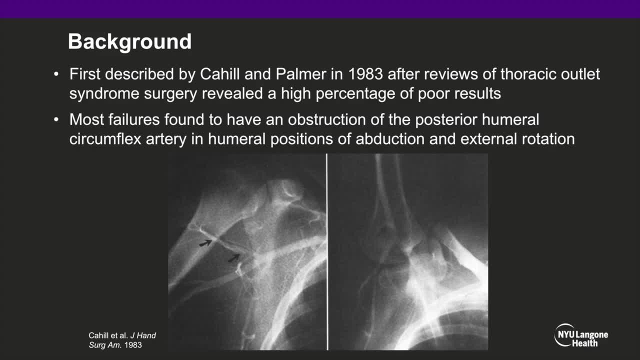 are compressed within the quadrilateral space. This condition was first described by Cahill and Palmer in 1983. after reviews of thoracic outlet syndrome, surgery revealed a higher than expected percentage of poor results. Most of the failures were found to have an obstruction of the posterior.